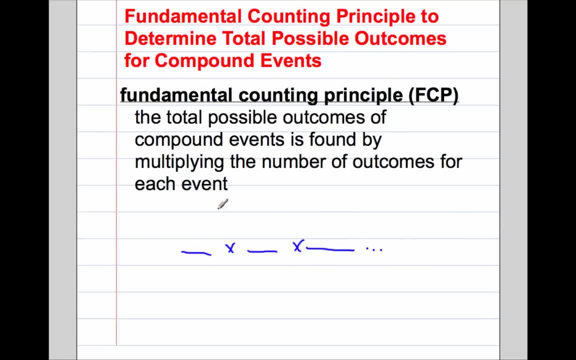 Alright, and if I had more events, I'd keep on doing the same exact thing, Alright, and that would. That would give me the total possible outcomes I should have, and then I can list the outcomes separately, as we did in our previous video on listing the possible outcomes. 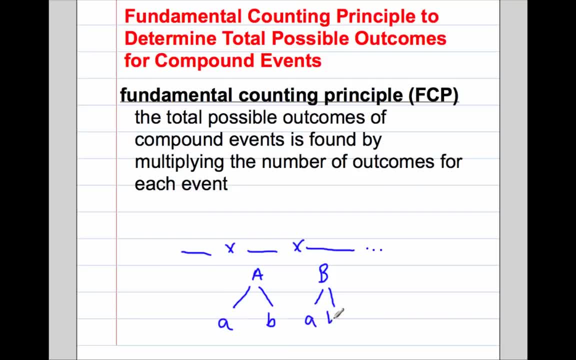 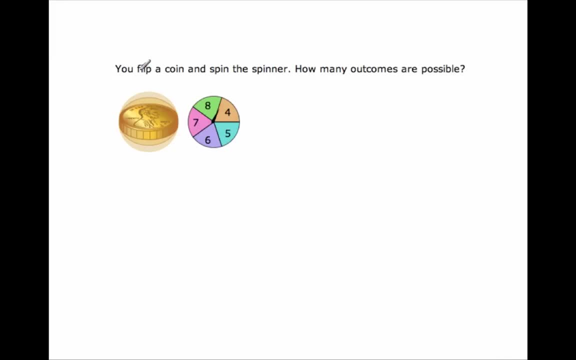 Alright, For compound events. Alright so, but in this video, all we're trying to do is determine how many, not. what are the outcomes? Alright, let's go to some problems to see how this works. Alright, you flip a coin. 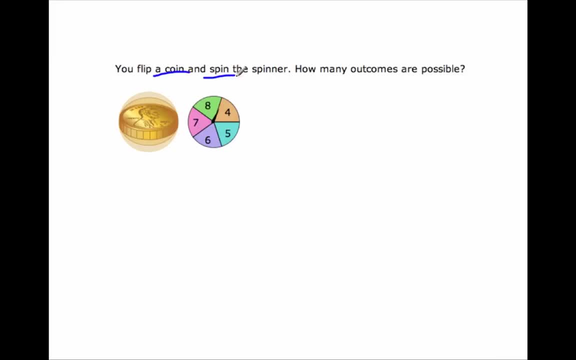 Flipping a coin and spin the spinner. So those are two different events. How many outcomes are possible? Well, flipping a coin, how many outcomes do you have there? Two It's heads or tails, And then how many outcomes do you have for spinning the spinner? 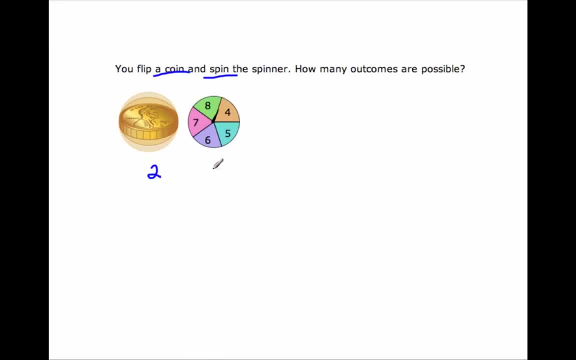 Let's count One, two, three, four, five different outcomes. So how many total possible outcomes do I have? Well, it's two times five, which is ten possible outcomes. Okay, and being precise, I wouldn't just write ten, I'd write ten possible outcomes. 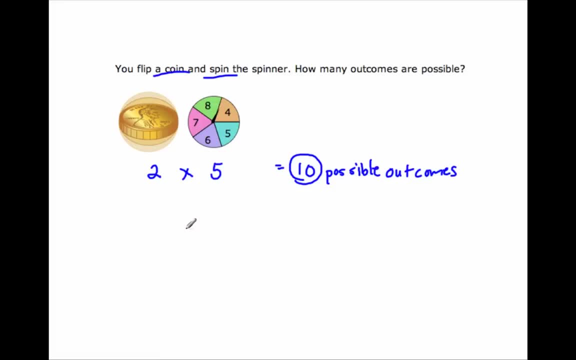 Alright. and then if I were asked- but this is not the task- if I were asked what are the outcomes, then I would look at the first event. What are the outcomes for the first event? Heads or tails? How many outcomes do I have for the next event? 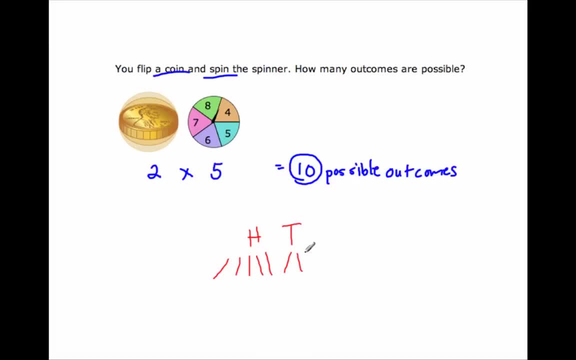 Five. so I'd draw five separate branches and then I'd list them. Okay, So I'd have eight, four, five, six, seven, Eight four, five, six, seven, And then I'd list them out. 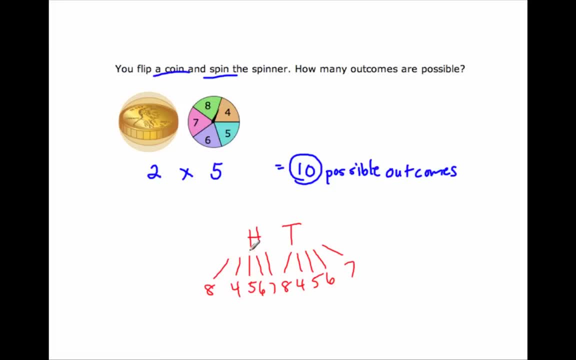 H-H, H-8, H-4, H-5, H-6, H-7.. T-8, T-4, T-5, T-6, T-7.. And those would be my outcomes, And if you can see, there are ten of them. 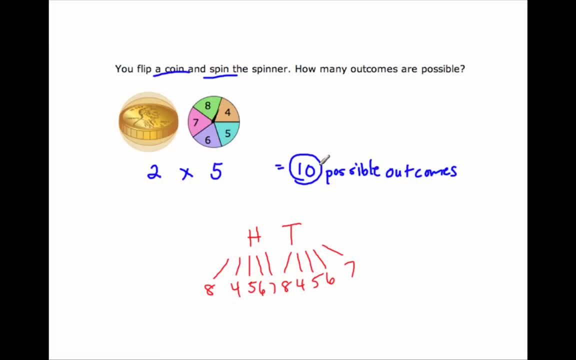 One, two, three, four, five, six, seven, eight, nine, ten possible outcomes. Alright, Alright, Just determining how many? Okay, Don't list them unless you're told to list the outcomes or ask what are the outcomes. 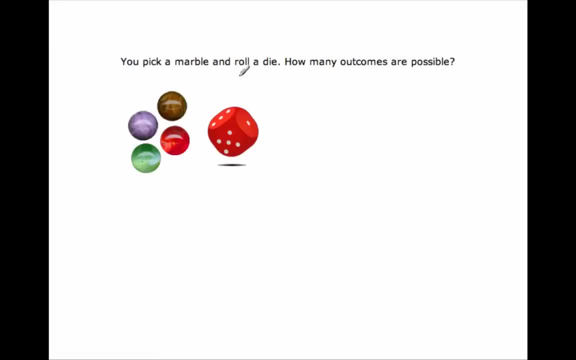 Alright, let's go to the next one. You pick a marble and you roll a die. Alright, How many outcomes are possible? Well, look at the marble. This is your first event. How many outcomes? One, two, three, four. 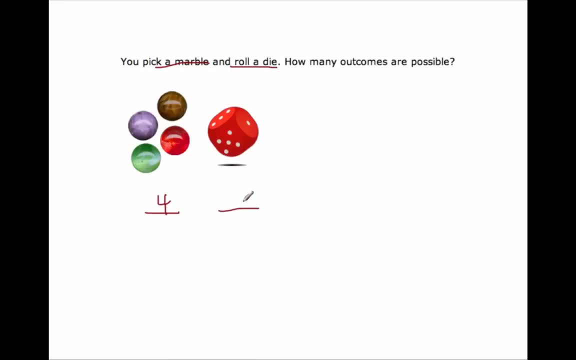 And look at your die. If you roll a die, there are six different sides, So you could land on six different sides And whenever you're determining outcomes, you multiply, Because if you look at your tree diagram, you'll see that you're actually just multiplying. 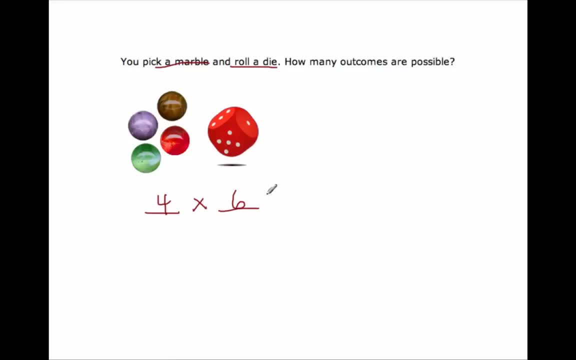 whatever you get here by that number. So four times six is 24.. Answer is 24 possible outcomes. Notice how this fundamental counting principle helps us to get the answer very quickly, as opposed to having to go through every single drawing to figure it out. 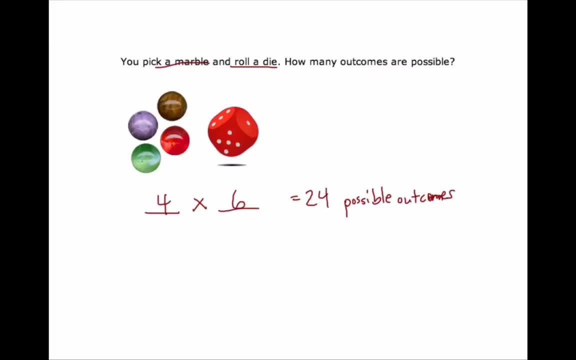 And then count later. It's a quick way, Nice math tool to help us. Alright, next You do the next problem and see if you can do this on your own and come back when you have the answer. Alright, you pick a marble and you roll a die. 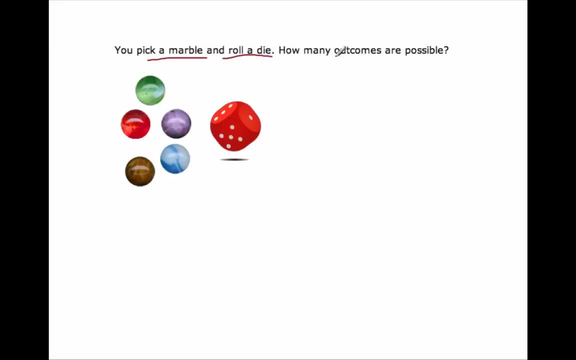 Those are two different events. How many outcomes are possible? Alright, so whenever I see this, I'm using the fundamental counting principle as a tool: One, two, three, four, five. For my first event of picking a marble And rolling a die, outcomes are six. 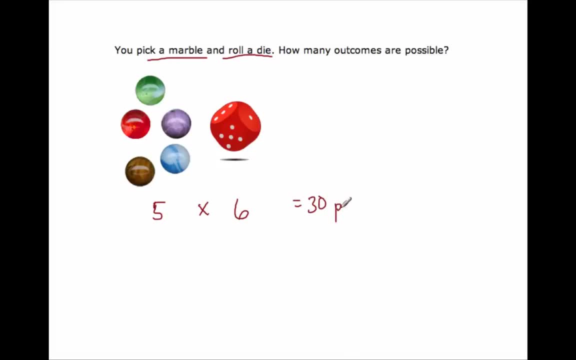 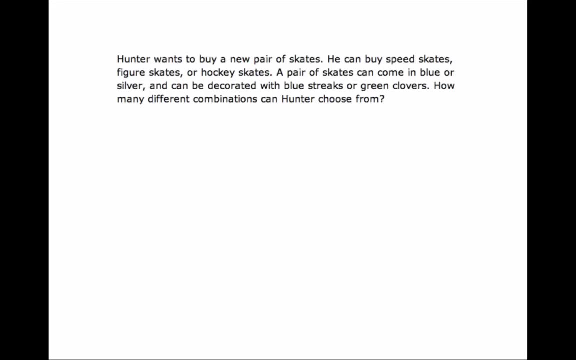 Five times six is 30. So I have 30 possible outcomes And the last one doesn't involve any pictures. so we have to make sense of this problem as we go through and persevere in solving it. Hunter wants to buy a new pair of skates. 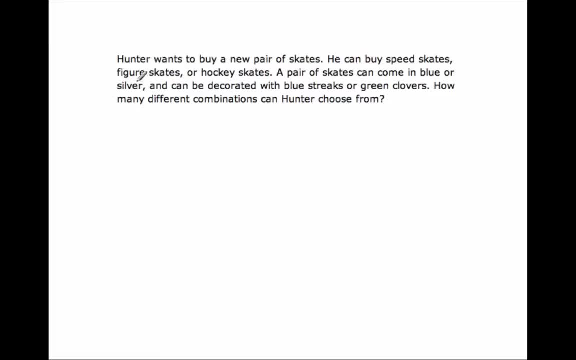 Alright. So first I'm going to buy a pair of skates, Alright. So Hunter wants to buy a pair of skates. I just know Hunter wants to go shopping for some skates. He can buy speed skates, figure skates or hockey skates. 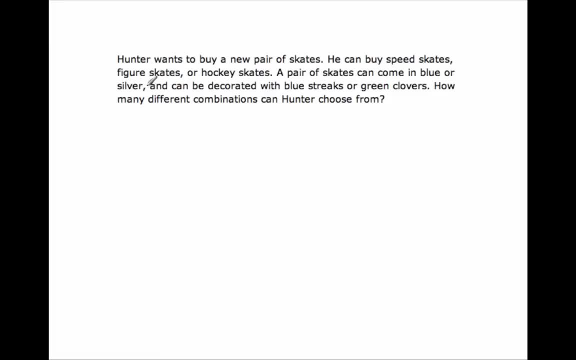 Alright, A pair of skates can come in blue or silver and can be decorated with blue streaks or green clovers. How many different combinations can Hunter choose from? Well, first I have to figure out what are my different events here.